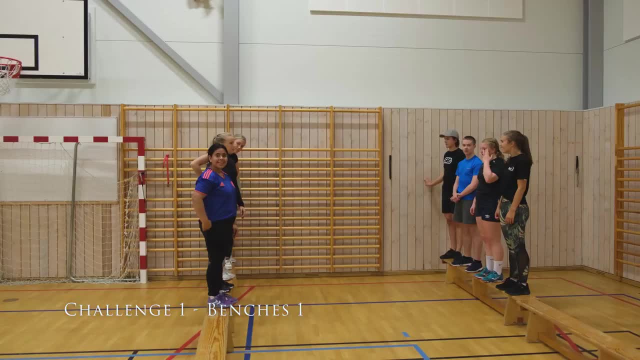 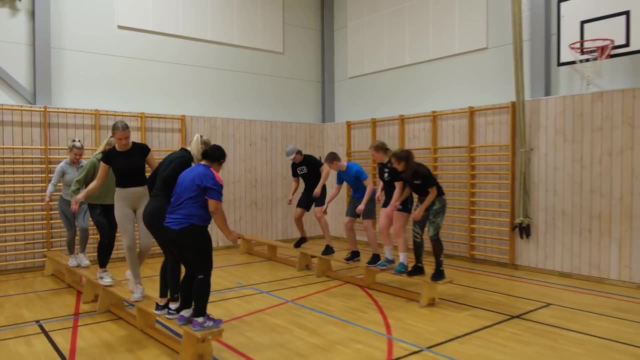 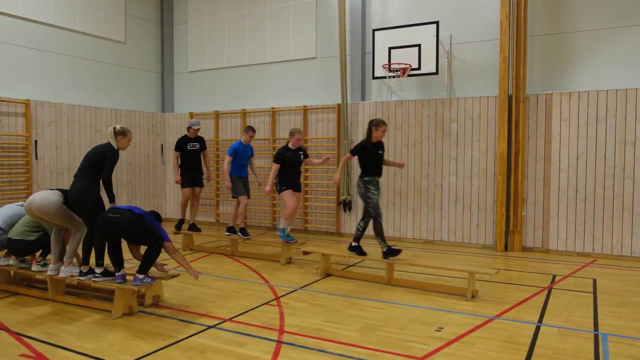 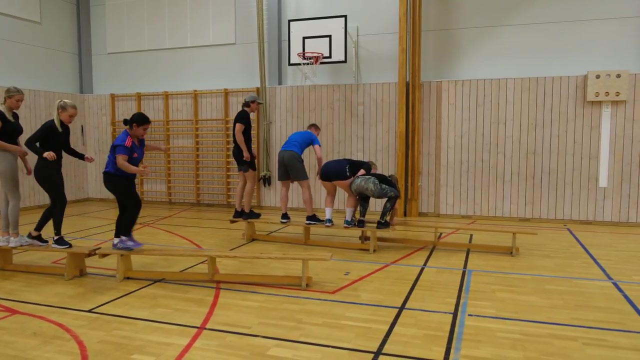 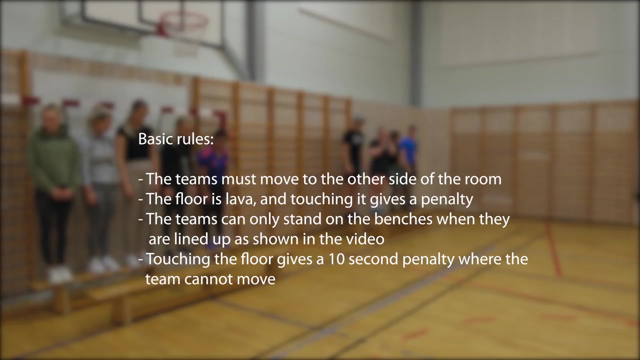 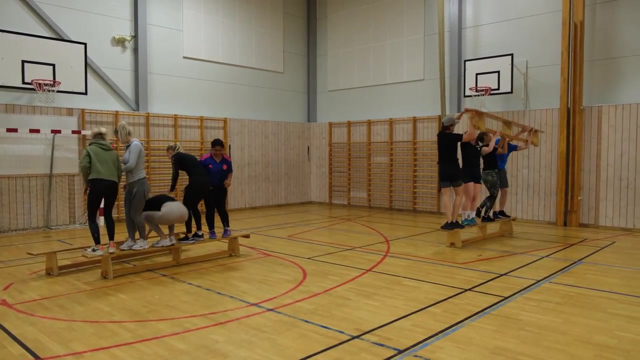 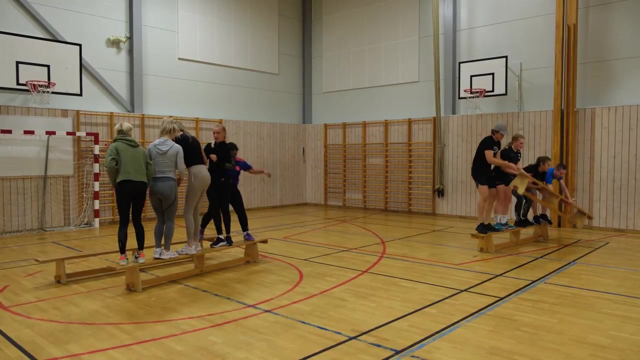 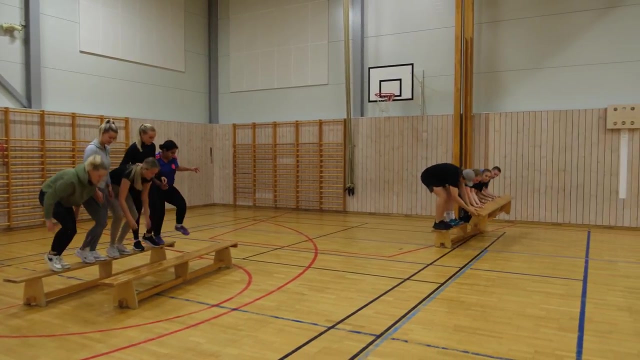 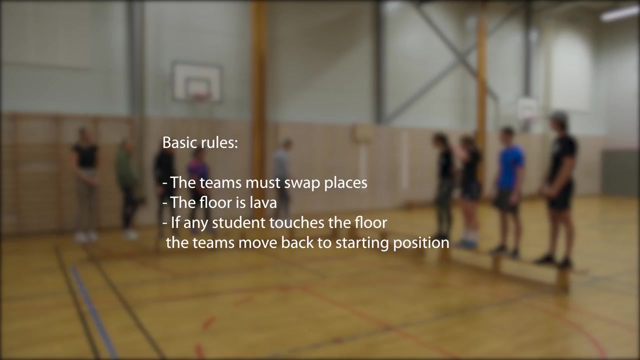 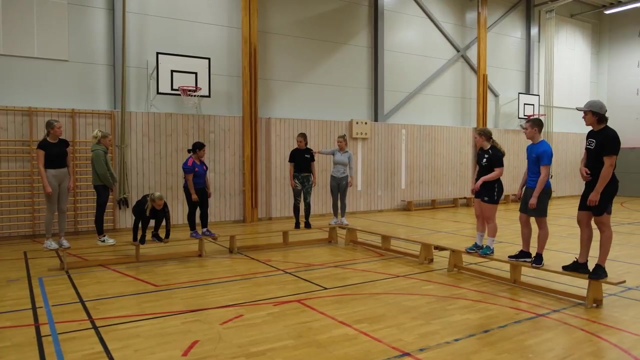 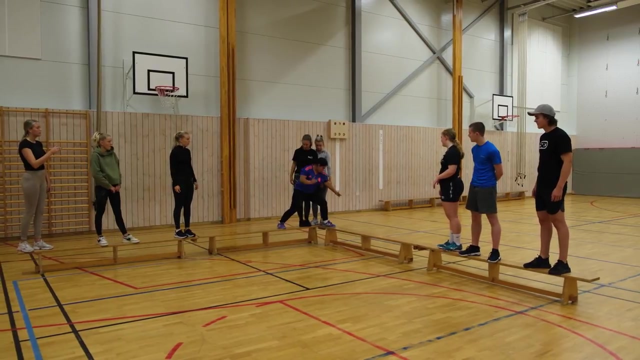 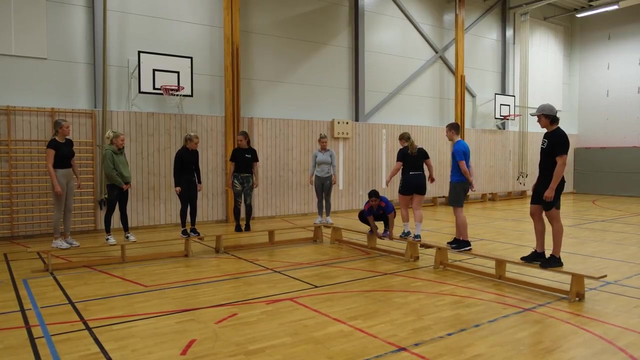 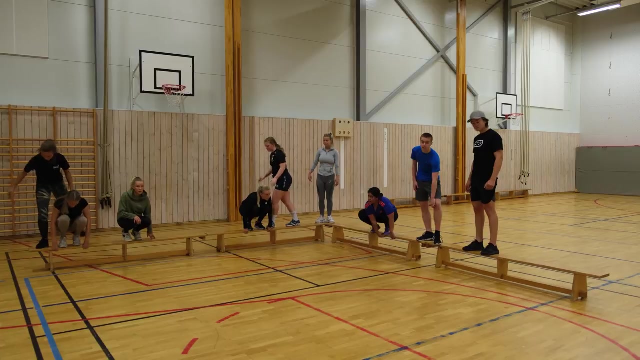 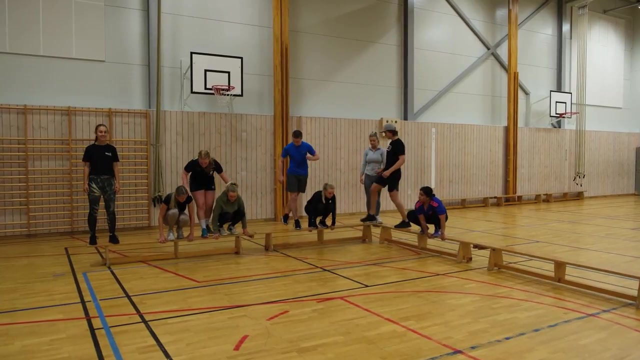 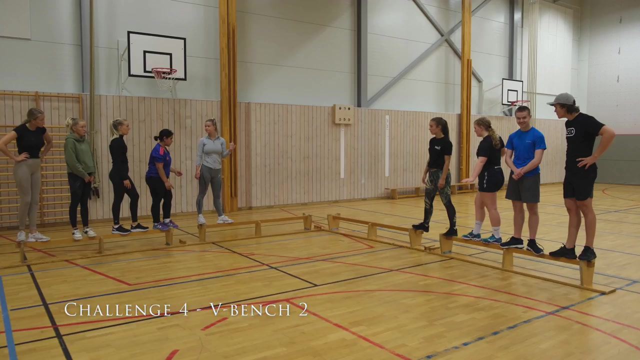 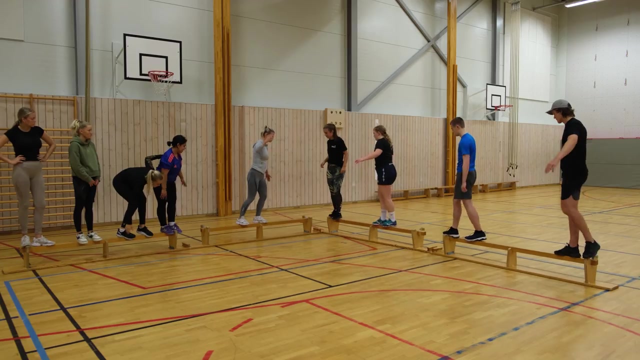 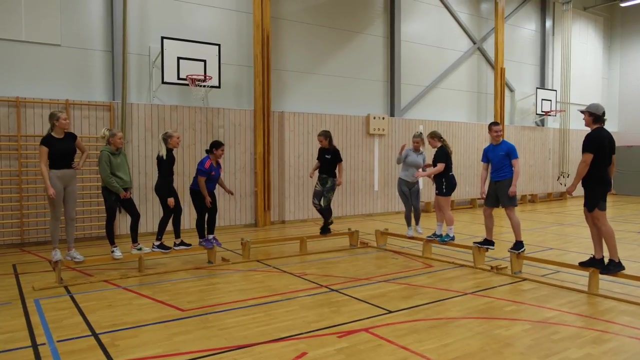 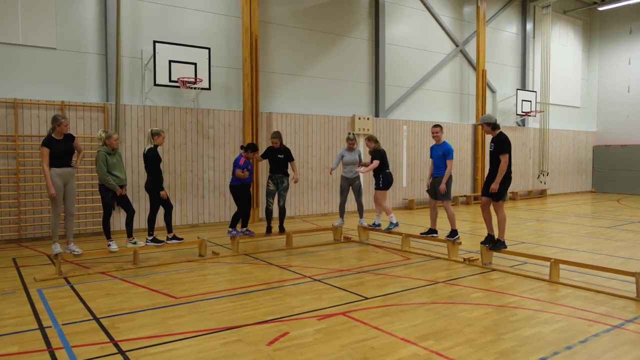 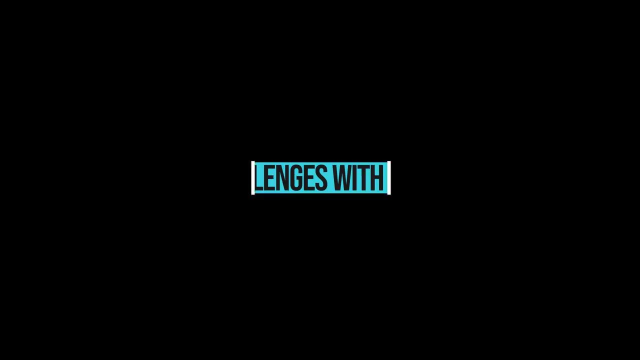 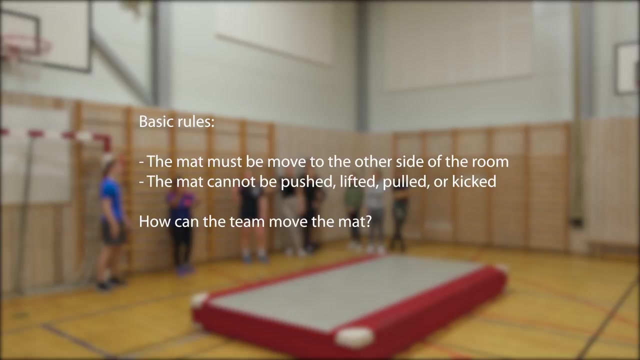 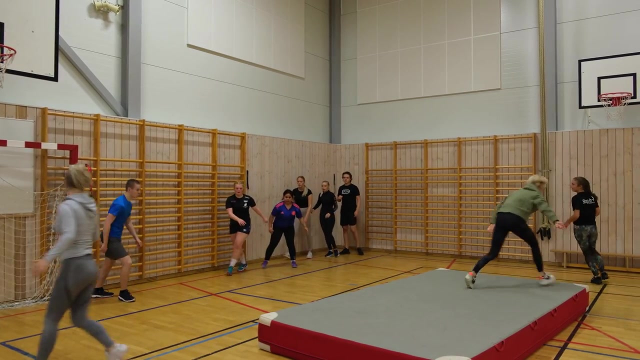 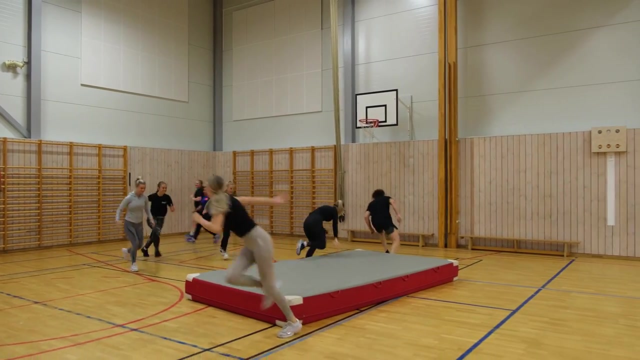 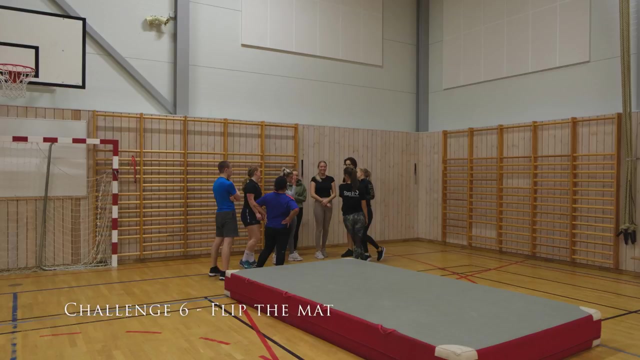 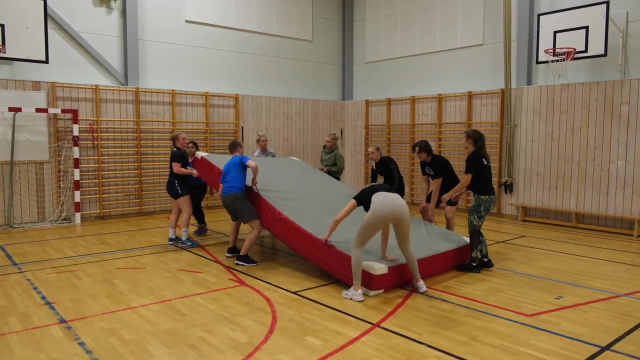 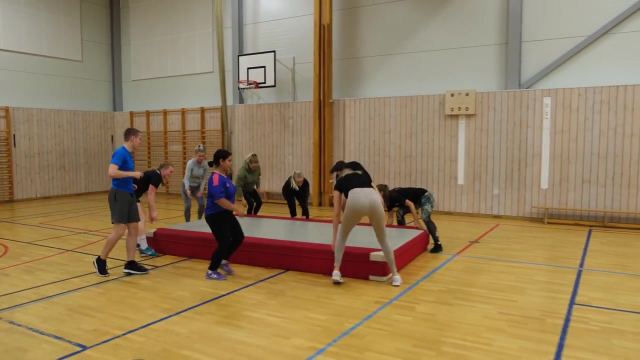 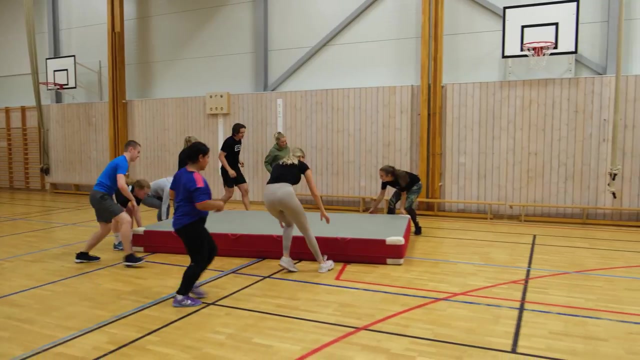 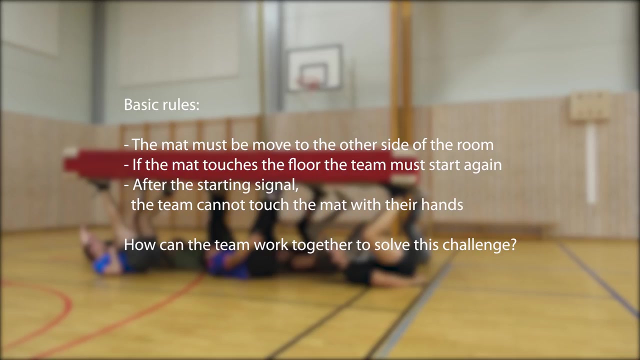 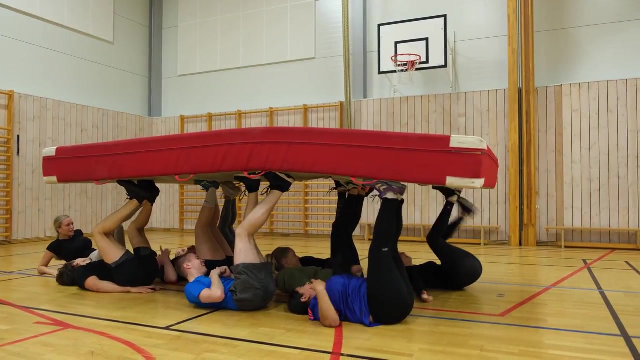 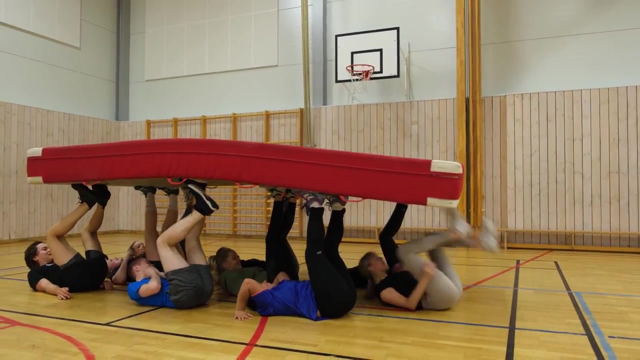 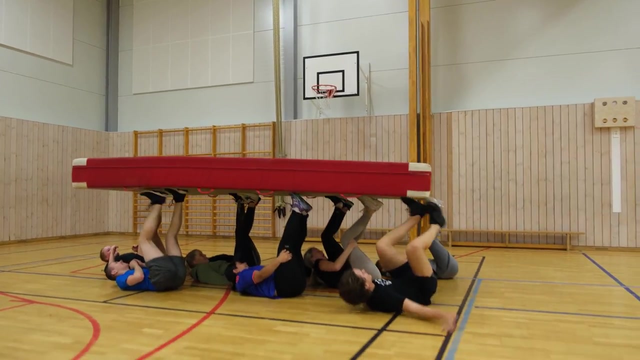 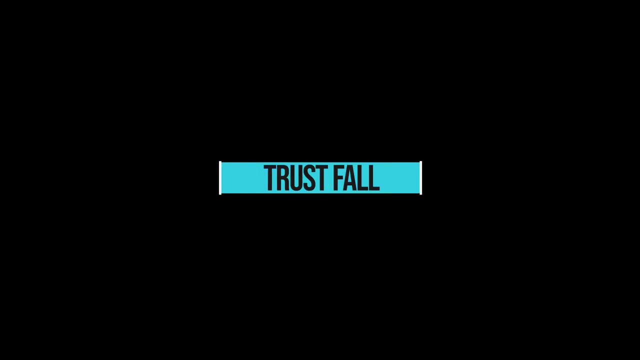 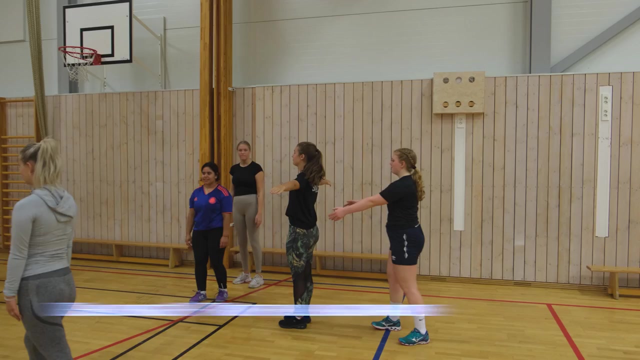 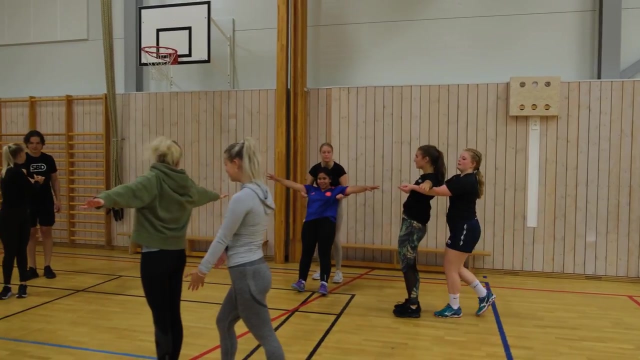 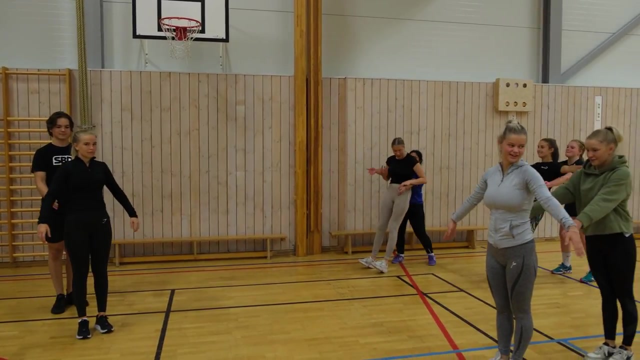 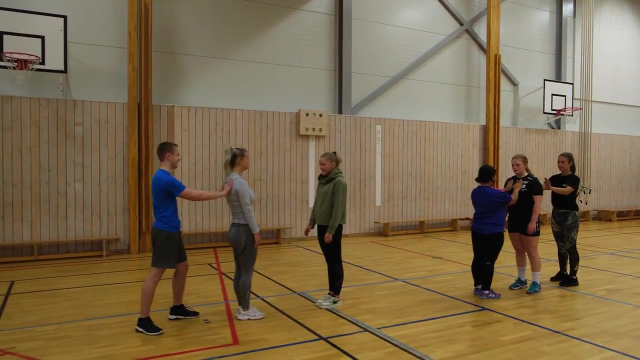 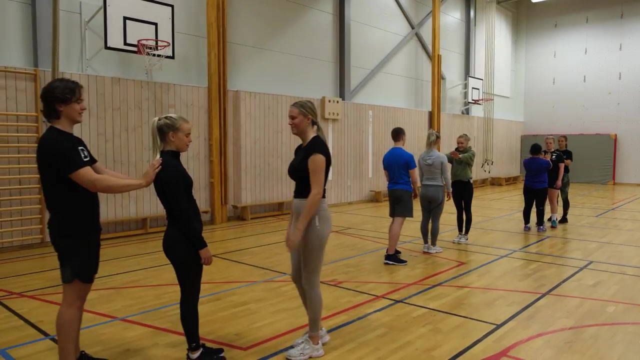 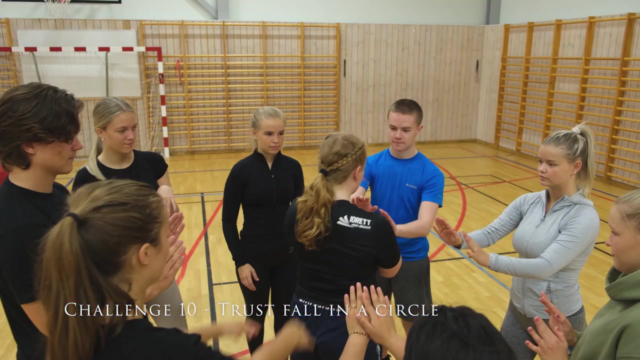 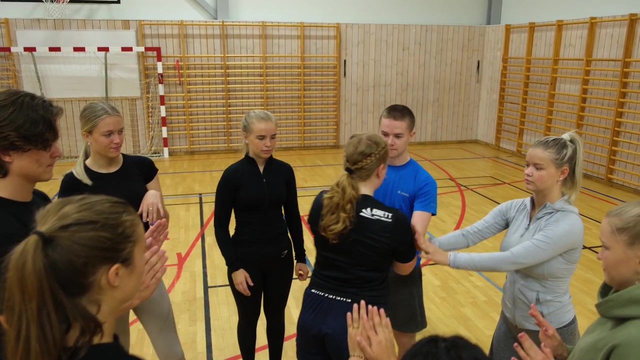 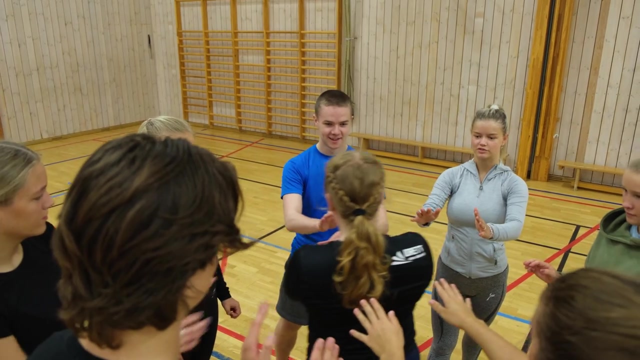 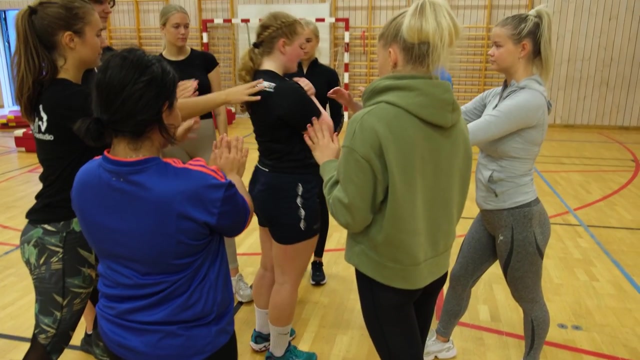 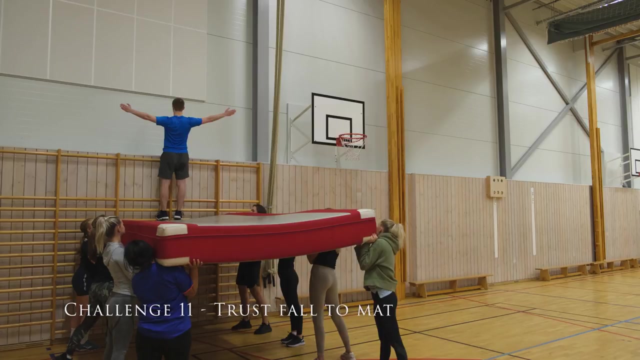 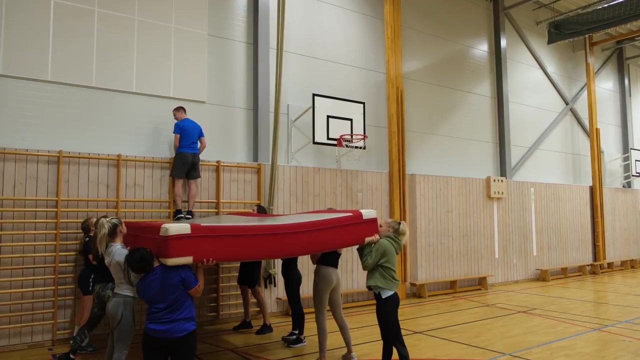 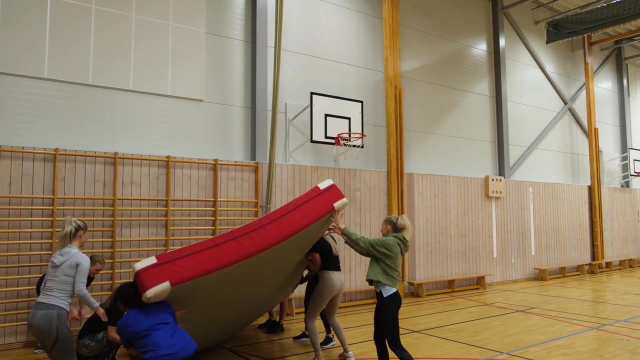 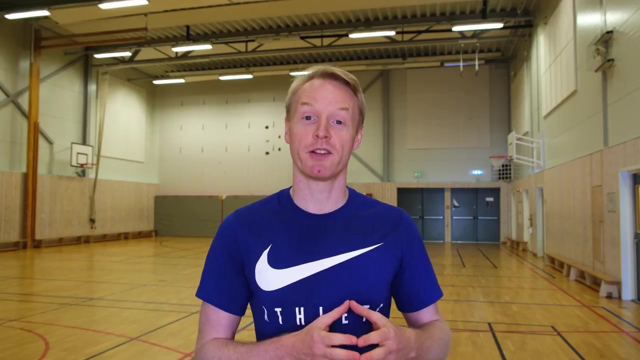 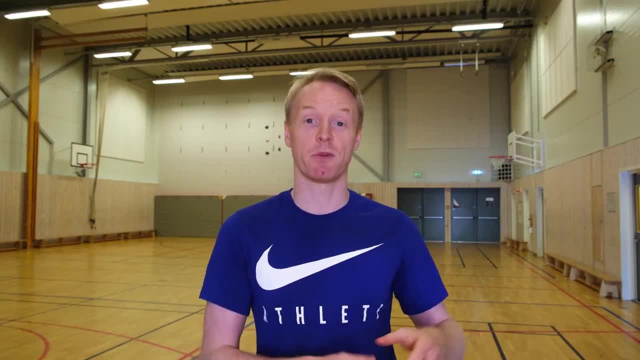 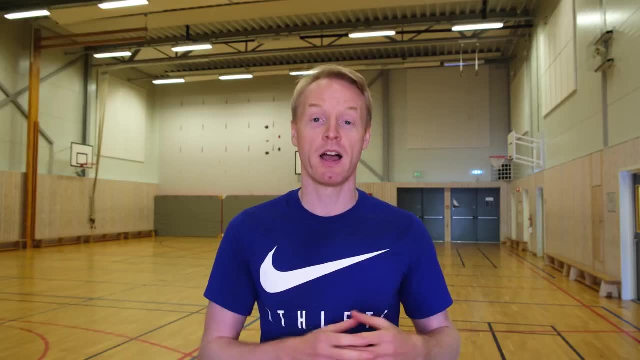 We have our students put out the equipment they need for the exercise, Then we tell them the set of rules that apply to this exercise And then we give the students one to two minutes to discuss in the group. how are we going to solve this problem and what solution are. 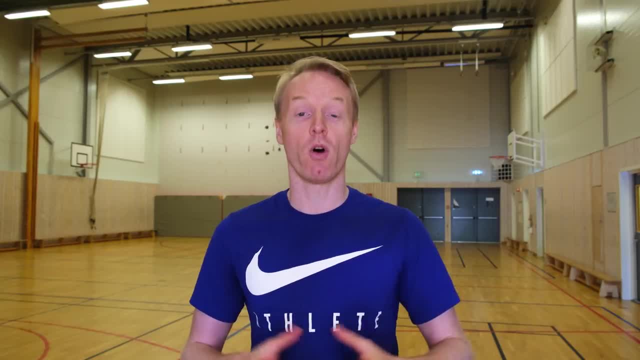 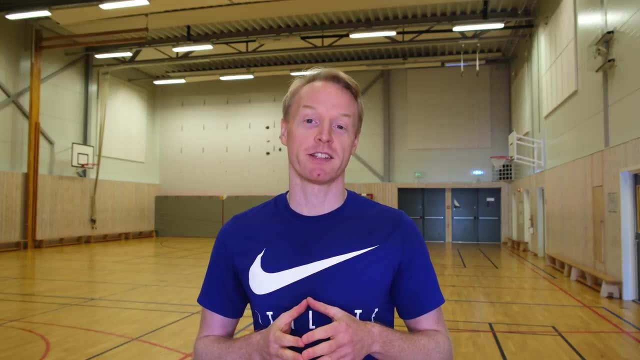 we going to use, And after the two minutes are over, all of the group starts at the same time. So these exercises are a great starting point for discussing important topics in physical education. We start off today by talking about cooperation. How does a group function? How do we make sure? 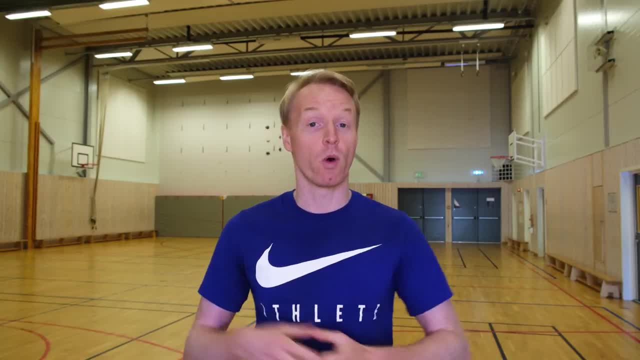 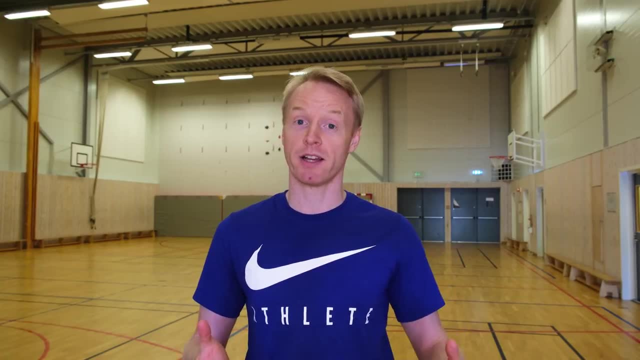 that all of the members of the group are included in the discussion. What can go wrong when we work in a group? I'll look at stuff that happens during the exercises and we'll talk about that with everybody. One of the teams may win and they'll be really happy. 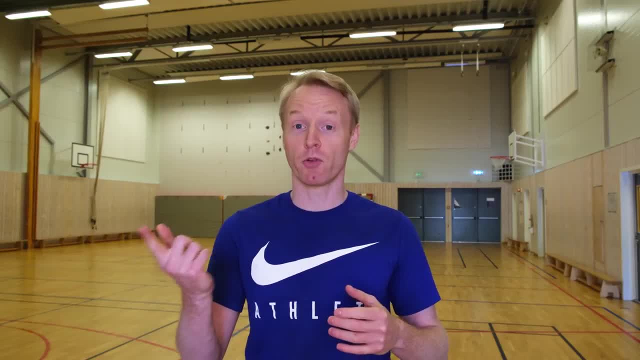 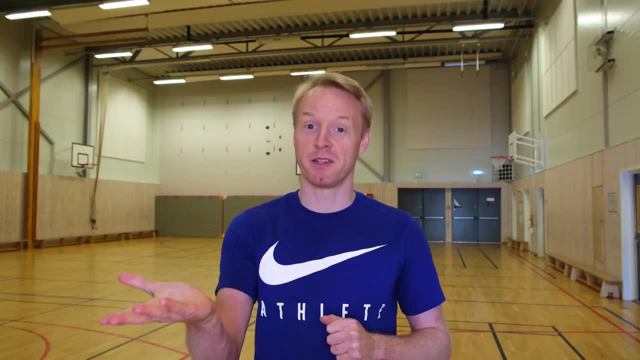 about winning, and maybe they'll start saying something about the other groups that haven't finished yet, And that's a good point to start discussing. What does it mean to be a good winner And what does it mean to be less of a good winner, And how does your? 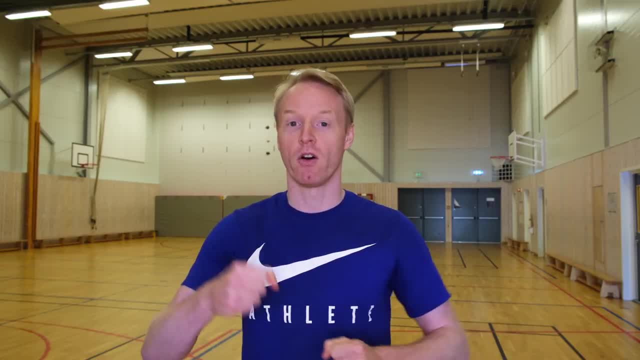 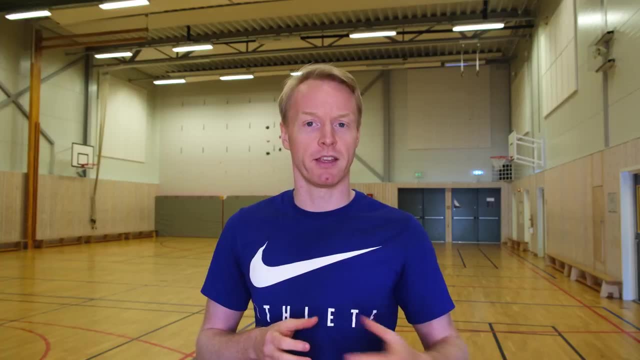 behavior affect the other students. if you behave in this way or you behave in that way, And then you have groups where students might get a little bit annoyed, Maybe some of the students will say something and maybe the person that is stepping down or not being able to do it is starting. 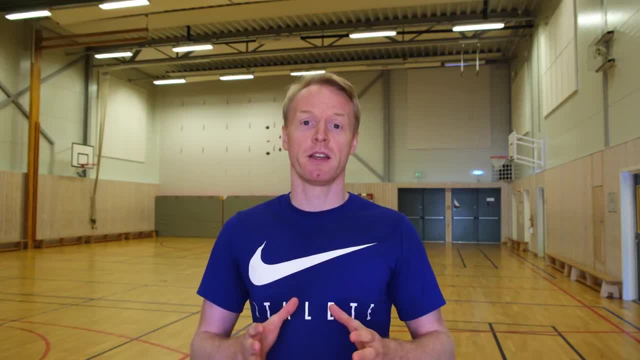 to feel really unwell, And that's a perfect point to stop and then think about. how does a group function? In physical education, you are supposed to be allowed to make errors, Otherwise you cannot grow, And it's the group's job to make sure that everybody. 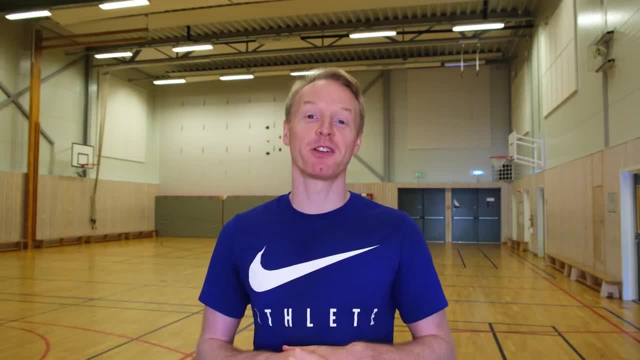 feels it is okay to make errors. I really enjoy doing these exercises with my students. We have a lot of laughs and it's a really good workout once the students get really into it. I hope you got inspired and I am excited to see if any of you try it out. 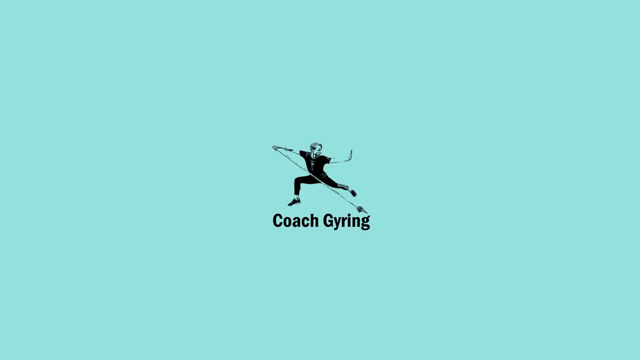 Best of luck. Music, Music, Music, Music Music.